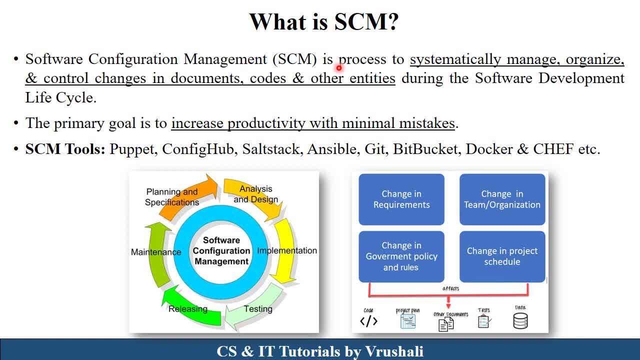 process is used. As per the definition, SCM is process. who systematically manage, organize and control all the changes in documents, codes and other entities in SDLC To monitor all these changes are necessary because it affects on your programming code, your project planning, then your testing data and other. 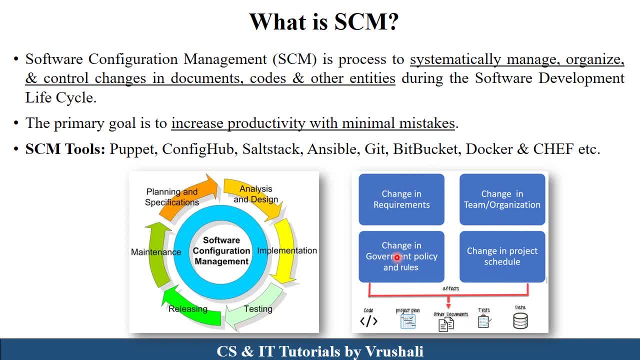 database To handle all this configuration items. there are different SCM tools are available, like Puppet, ConfigHub, then Solstack, Ansible, Git, Bitbucket, Docker. These tools are used by the configuration manager to handling all the configuration data. The primary goal of SCM is: 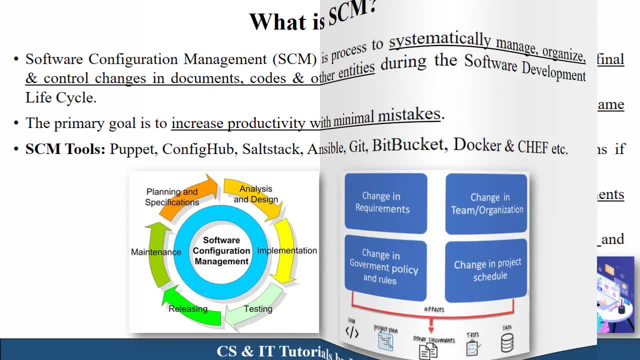 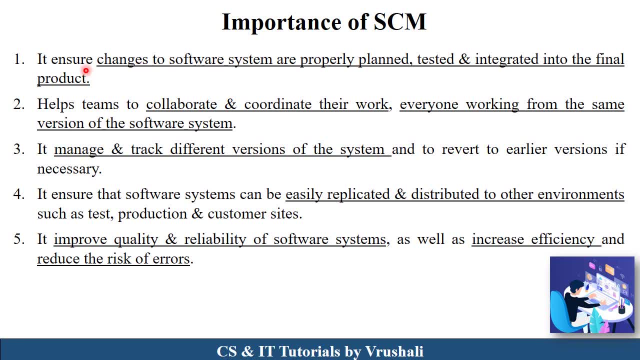 to increase productivity with minimal mistakes. Now the next topic is importance of SCM, and the main importance is configuration manager ensure that all the changes occur in software project are properly planned, tested and integrated into the final product. It also helps software team members to collaborate and coordinate their work. Let's take one example. Suppose there are new. 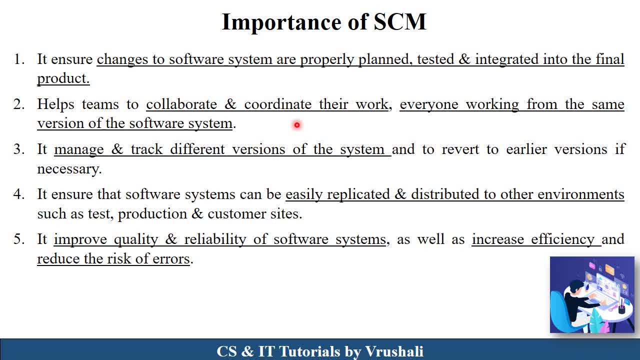 WhatsApp updates are available, So at that time you update your WhatsApp from the Google Play Store, So at that time there are new features are available, right? So this SCM process manage and track different versions of particular software system. They also ensure that everyone working from the same version of software system. 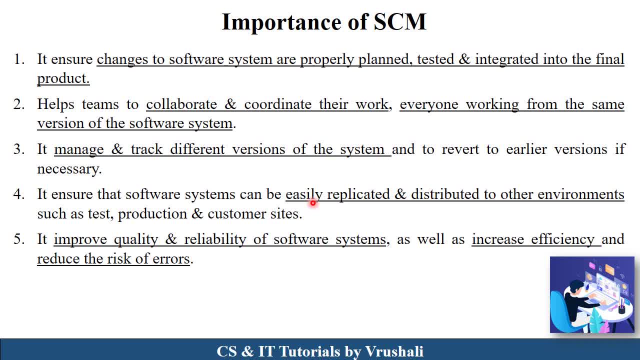 SCM also help in deployment phase of software development lifecycle. They maintain environment on the client side while developing a particular product. Basically, it improve quality and the service life of those software system. It also increase efficiency and reduce the risk of errors in particular software project. So this is the importance of SCM in software engineering. 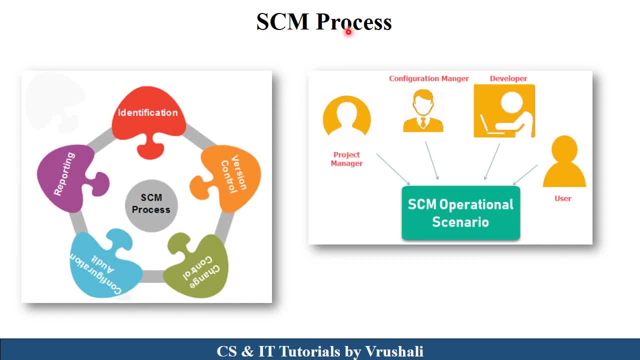 Now the next topic is SCM process. As per your exam point of view, this is one of the most important topic. There are total five steps in SCM process, like identification, version control, change control, configuration audit and reporting. This SCM process are handled by two main components. The first one is called the New SCM process. It is a process that helps the number one ECM data of your system. 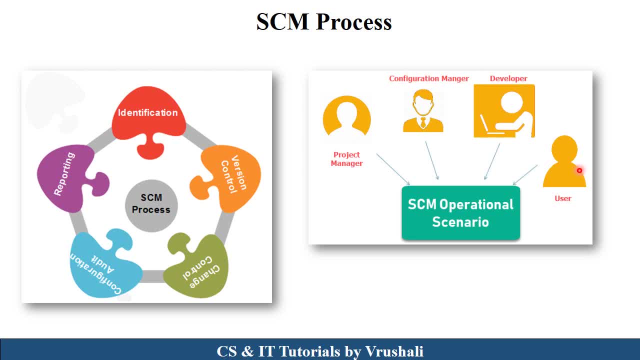 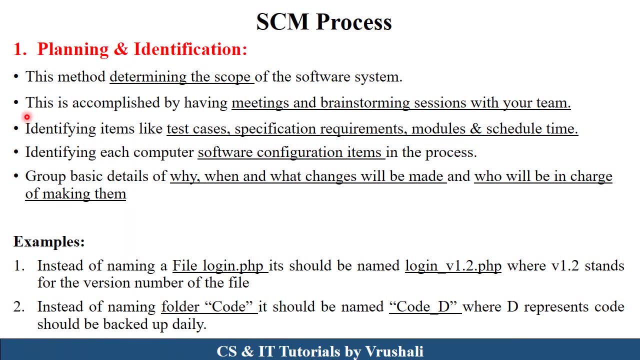 by the project manager, configuration manager, developer and the end user. Now let discuss SCM process in detail. Now the first step of SCM process is planning and identification. Here configuration manager identify the scope and objective of particular software project. For that purpose they arrange meeting, group discussion, brainstorming session with your 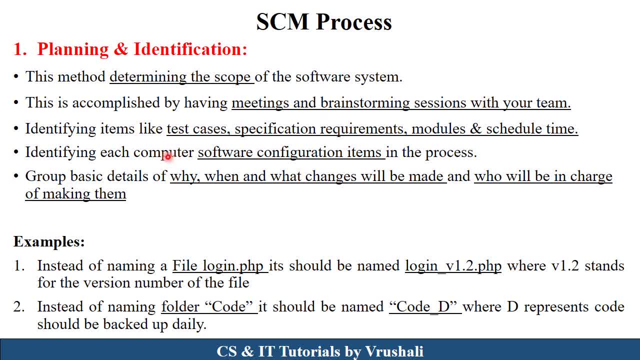 software team and different stakeholders. Configuration manager identify different test cases, requirements, different modules and schedule time of particular project. They also identify software configuration items means which type of hardware resources, software resources and human resources are used in particular project. Basically, they maintain a details of why, when and what changes will be occur in the 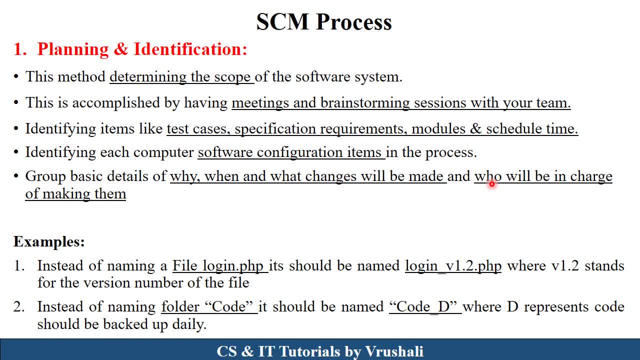 particular project and by whom this all changes are performed. They identify and analyze all these details. They also mention proper naming convention to each and every file. See here: instead of naming a file, loginphp, you should give a file name: login, v1.2.php. 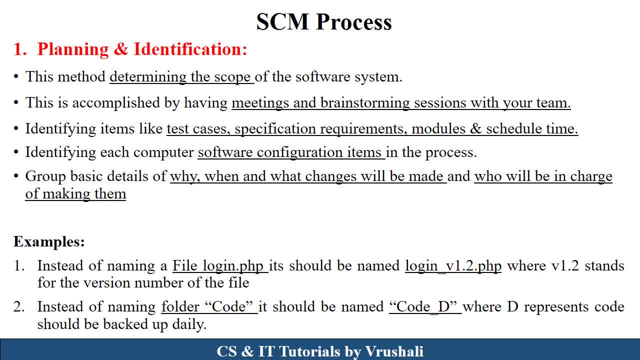 Here v1.2 stands for version number of file. See Every time new features are added in particular project. So also change the name of that particular file. That is version 1, add new features. that is version 2.. Again, add new features. that is version 3. in this way: 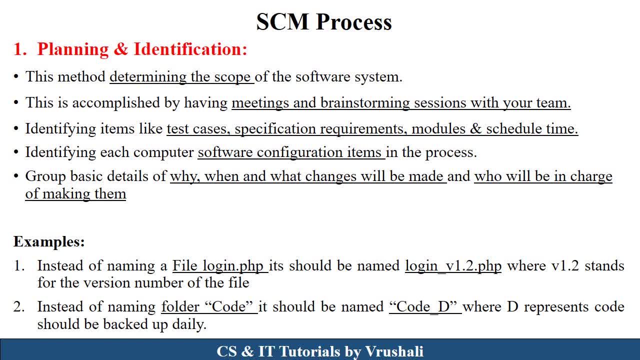 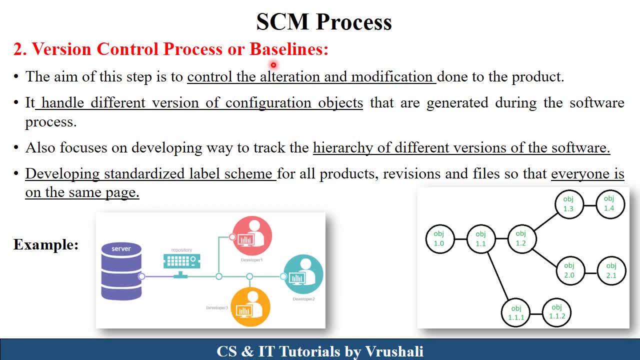 So mention proper naming convention to each and every files and the folders. Now the second step is version control process or baseline, See SCM process. handle different versions of configuration objects and the particular product: See here in this diagram. Suppose: developer 1 work on whatsapp v1.1 file. that is first version of file. 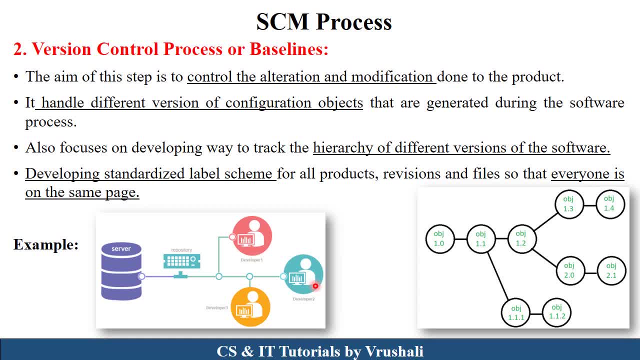 Now developer 2 add some extra features in particular product. Now they mention a file name. whatsapp v1.2 means second version. Similarly, developer 2, developer 3 edit that particular file. also add some extra feature in that file. Now developer 3 give the file name whatsapp v1.3.. 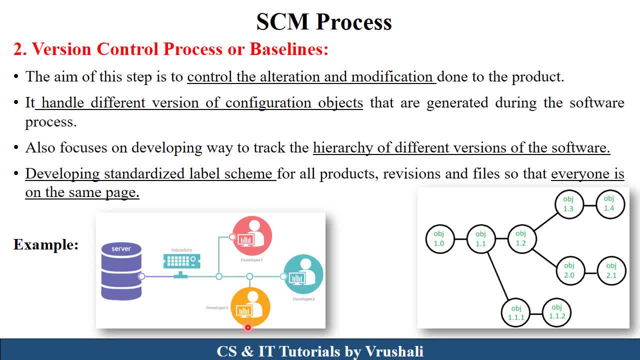 Means third version of that file. Now this last updated file stored into this repository And multiple stakeholders use this latest or updated version of file. So these process are handled by the configuration manager in SCM process. They control the alter, modification and storing all this latest version file into the repository. 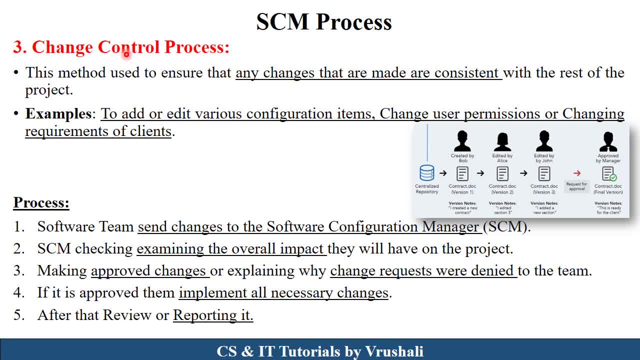 Now the next step is change control. See There are various changes are occur at each phase of SDLC: The changes related to the add or edit various configuration item, changes related to the user permission or sometimes changes related to the client's requirements right. 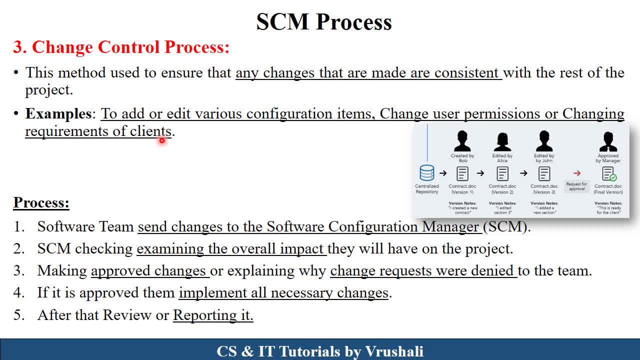 Now when there are changes are available. So what is the process? See here: Suppose customer want video call this new feature in particular project, right, So this changes is there. Now software team send this particular changes to the software configuration manager. Now software configuration manager check that overall impact of that particular change in. 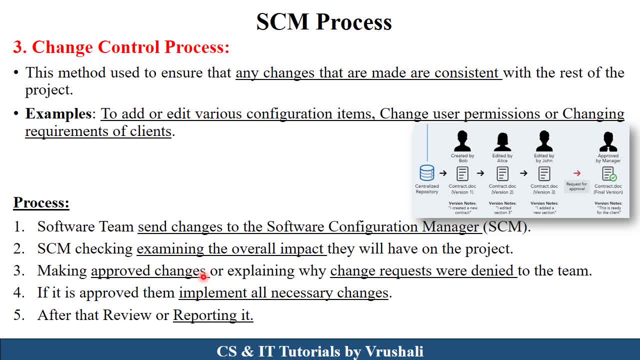 your project. After that, they approve those changes or denied those changes. If particular changes affect on your project or there is a wrong impact on your project, So configuration manager denied those changes. Otherwise they approve it: See Software configuration manager. approve those changes. 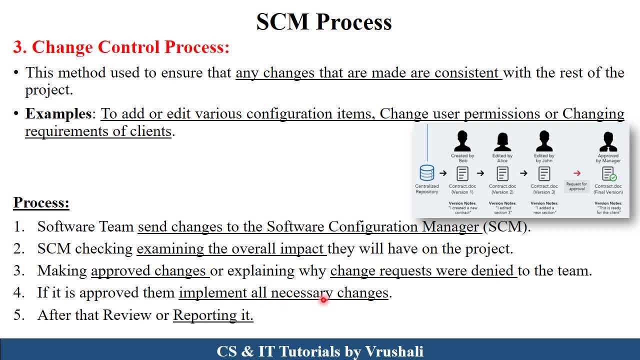 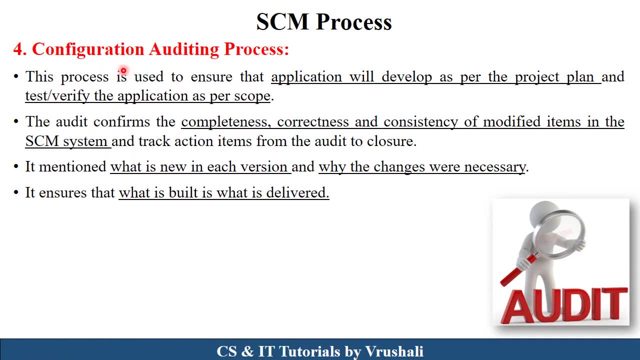 So implement all the necessary changes by the software developer and mention all these changes into the document. So this is called as change control process. So basically all the changes are approved by the software configuration manager. Now the next step is configuration audit process. So basically configuration manager here identify that all the changes are properly developed. 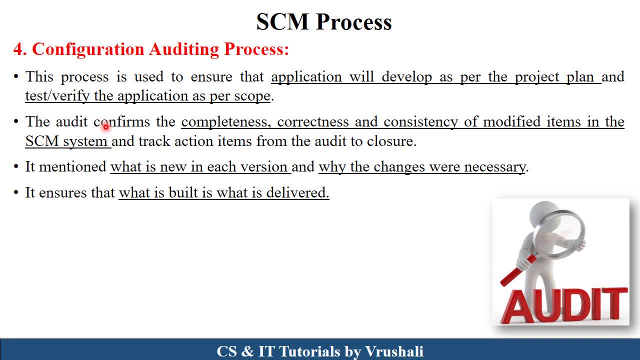 or not. They check that or they audit that- all the completeness, correctness and consistency of modified or changeable items in software configuration process. They also mention that what is new in each version and why the changes are necessary. They audit and verify all this complete process and maintain a document accordingly. 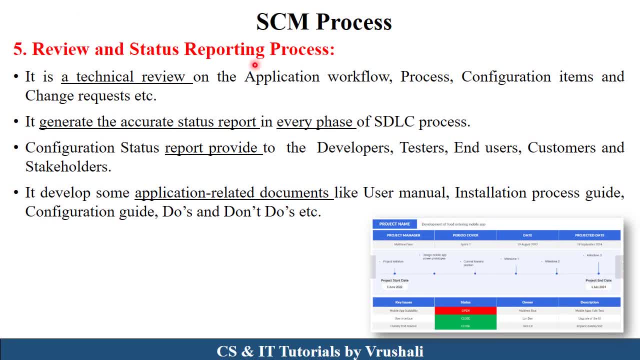 Now the last step is review and status reporting process. Basically, Configuration manager takes some technical review of each and every module in particular project. They take a review on application. workflow means complete workflow of your process, from start to end, various process and modules. configuration items means related to software and hardware. 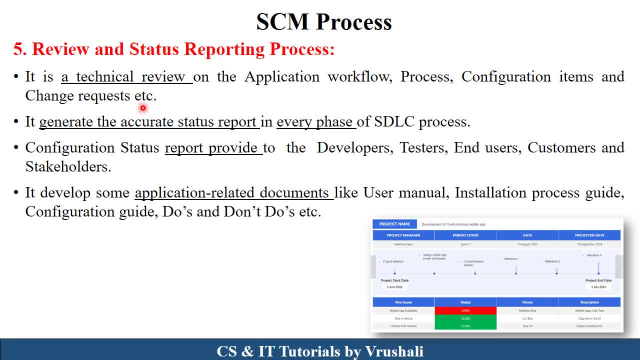 resources are properly used or not, and all the changing request of the client. They take a review of this thing and mention all these details in documents. Now This, This report, provided to the developer, tester, end users, customers and stakeholders. They check that your complete project is developed as per the customer requirements. 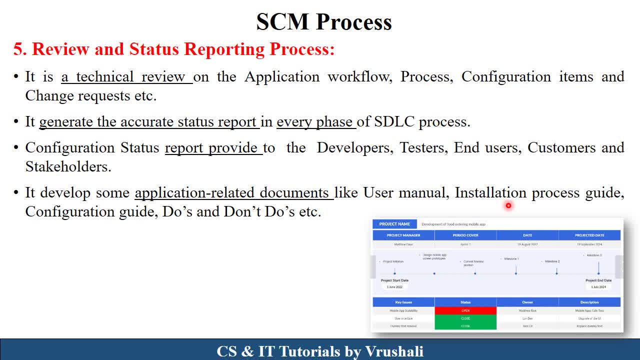 They also mention some user manual: installation process guide, configuration guide and do's and don'ts guide. See here: Suppose, when you buy a washing machine, So at that time there is a user manual, is there? this user manual mention everything: how to install washing machine. 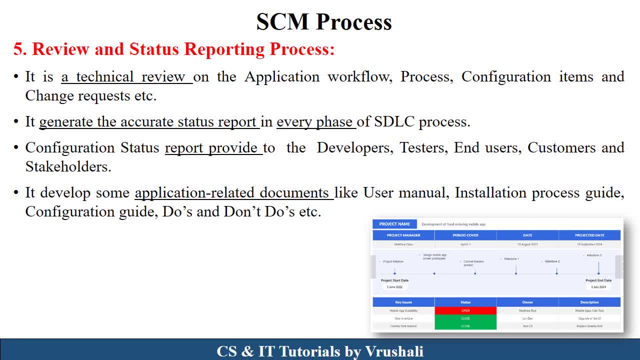 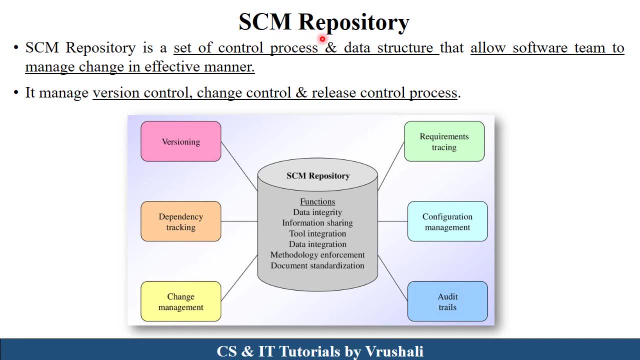 And how to use washing machine do's and don'ts related to the washing machine right. So this is called as review and status report. This is developed by the configuration manager. This is the last step of SCM process. Now the next topic is SCM repository. basically, SCM repository is a set of all control process. 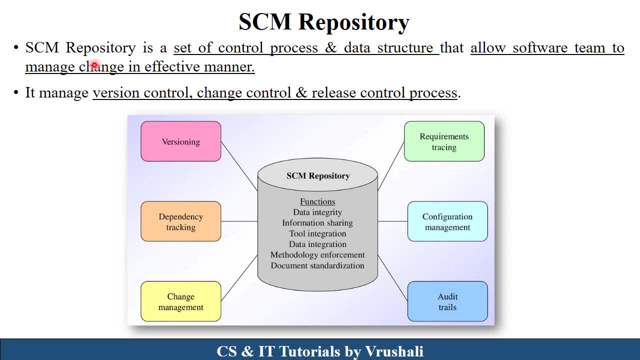 and data structure which allows software team to manage all the changes in effective manner. See here In this particular diagram. this is a SCM repository. there are total six tools are used, like versioning, dependency tracking, change management, requirement tracing, configuration management and audit trails. These are the six tools are used in SCM repository. 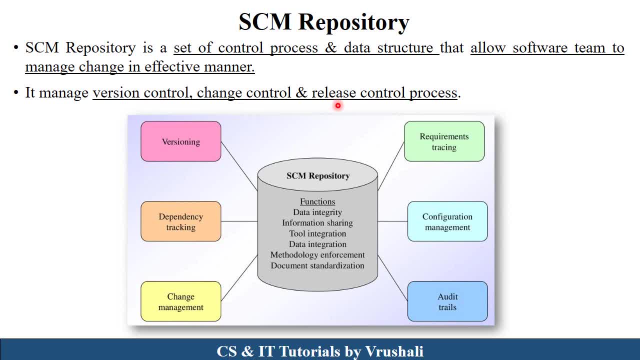 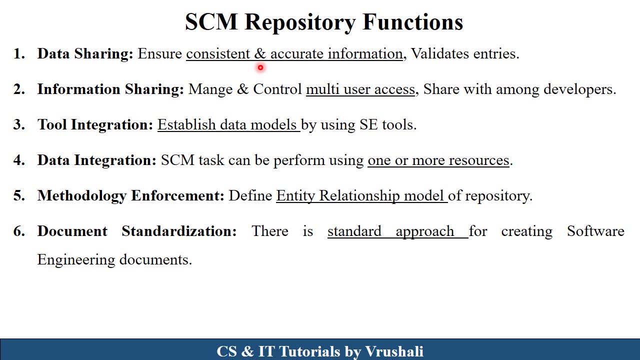 They manage version control, change control and release control process. Now these are the different functions of SCM repository. Now let's discuss The functions and tools in detail. Now why SCM repository is used in particular SCM process. basically, SCM repository is centralized database. all the changes are performed and after that stored these changes or updated. 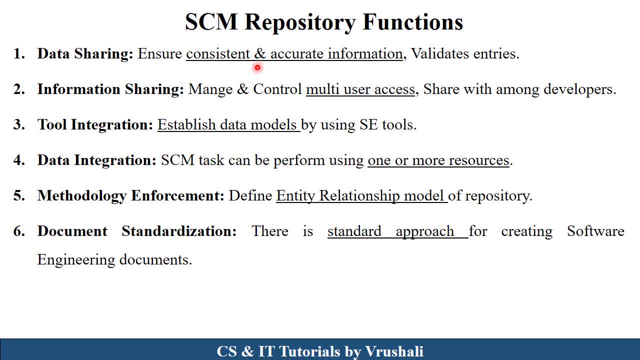 version file into the SCM repository. The first function is data sharing. means this SCM repository: ensure that all this information are consistently and accurately shared With all the stakeholders. then information sharing: multiple user access latest version of file from this repository. then tool integration: here SCM repository use different tools for. 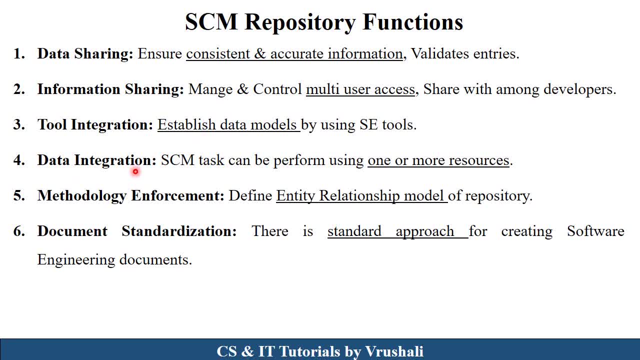 version control change control purpose data integration- here one or more resources- means different software resources, hardware resources, then different programming languages, database framework. So integration of all those things while developing a particular project. So this is the first function of SCM repository. Then tool integration: here SCM repository use different tools for version control change. 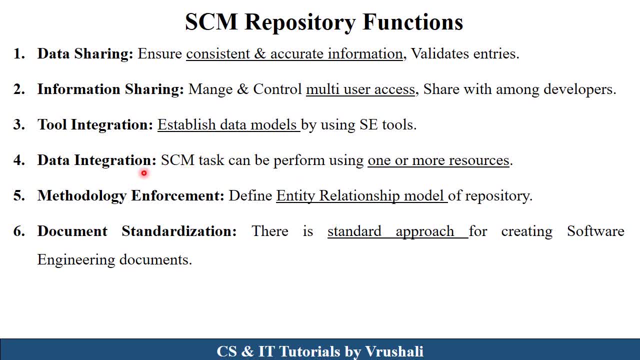 hardware zone of SCM repository, so they maintain this thing. next one is a methodology and for in enforcement. here the defined entity relationship model means while developing a particular project there are different modules, are there right and now there is an inter relationship between each and every module and also there is some authorization process. 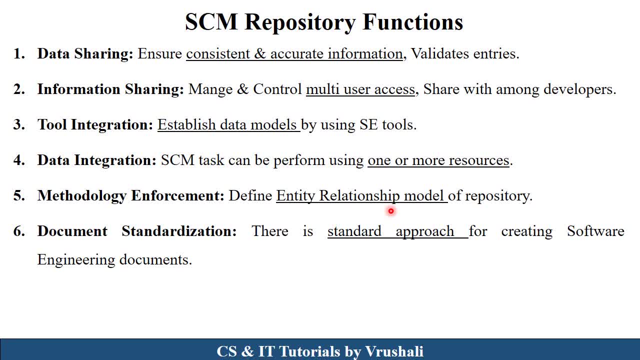 Let's take an example of college management system. there are, suppose, three module: student, teacher and HOD module. so this, all three modules, are interrelated with each other: student module used by the user. student teacher model used by the teacher. hod model used by the hod. also right, so this is called as entity. 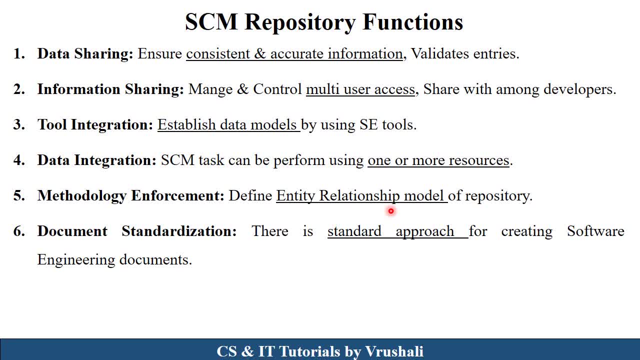 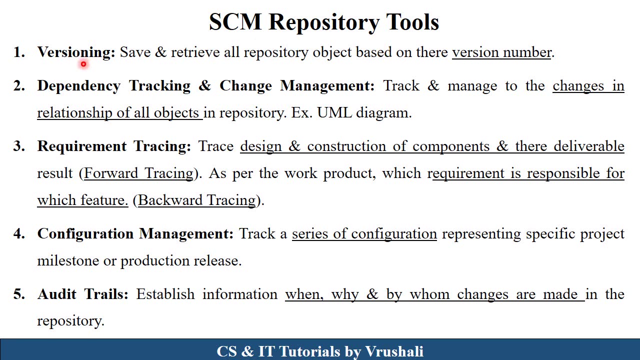 relationship model means which type of modules are there, what is their functionality and used by the which stakeholders. this is called as methodology enforcement. the next one is a document. standardization means everything have mentioned in document, in particular standard approach. so this is a scm repository function. now the next is scm repository tools. the first 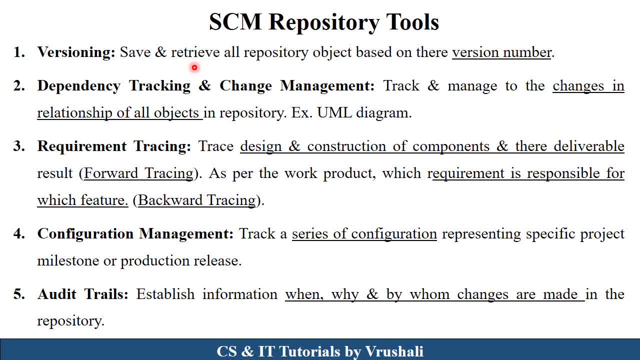 tool is versioning: see. as we discussed earlier, there are various versions of particular product and particular project. so this versioning tool mention all the version numbers of particular file as per their creation date. next one is a dependency tracking and change management: see as per the customer requirement. there are.